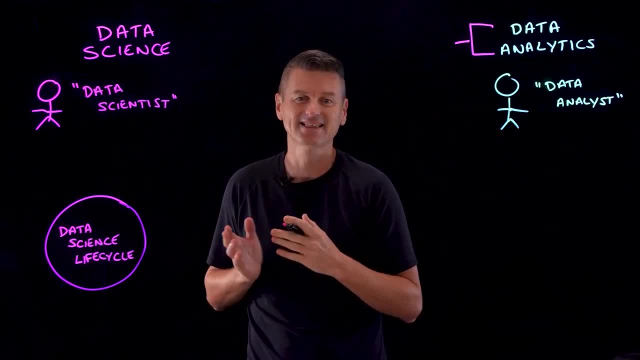 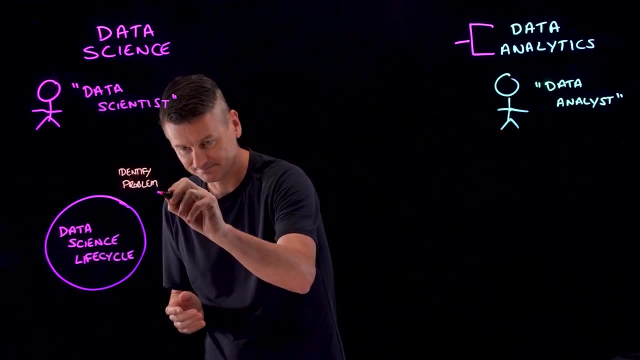 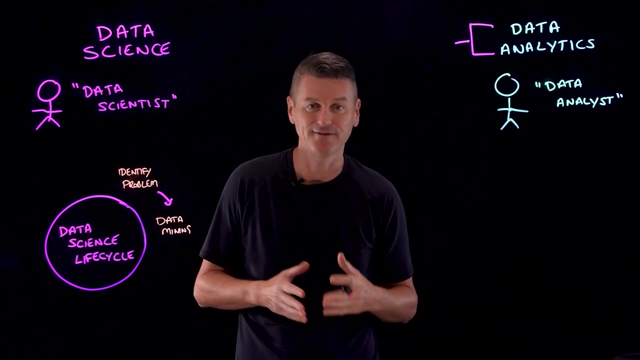 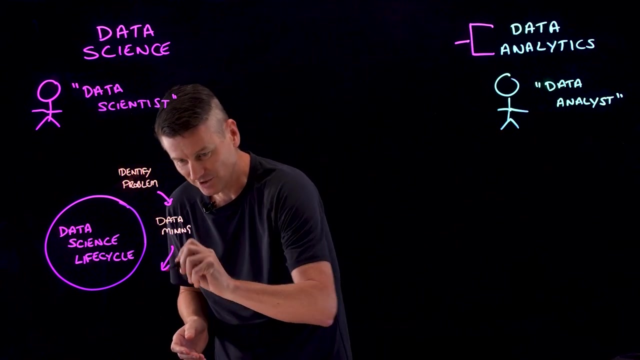 science life cycle, which usually follows seven phases. So first is to identify a problem or an opportunity. Then the next phase is data mining, which is to extract data relevant to that problem or opportunity from large data sets. Now that data will likely consist of a bunch of redundancies and errors, which is fixed in the next. 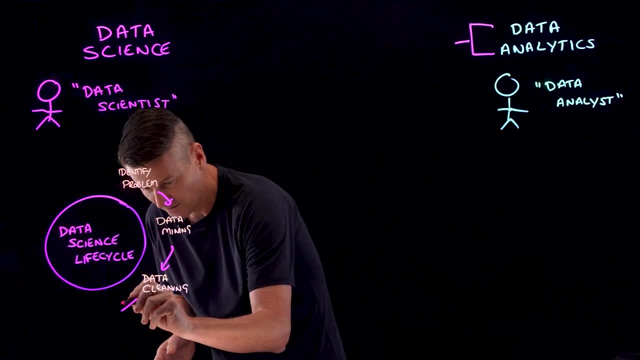 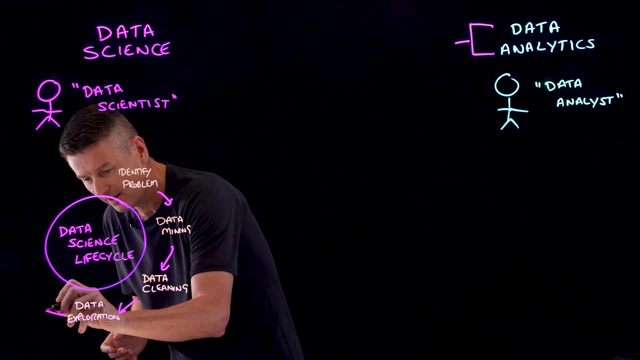 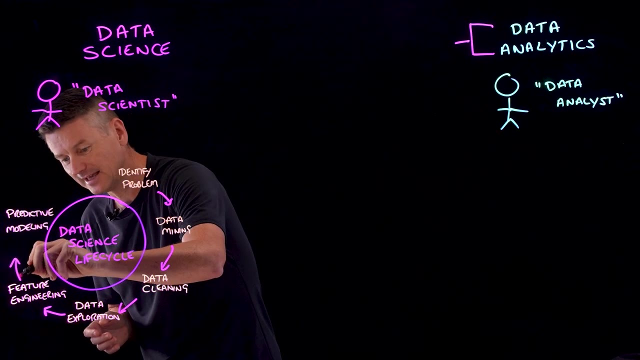 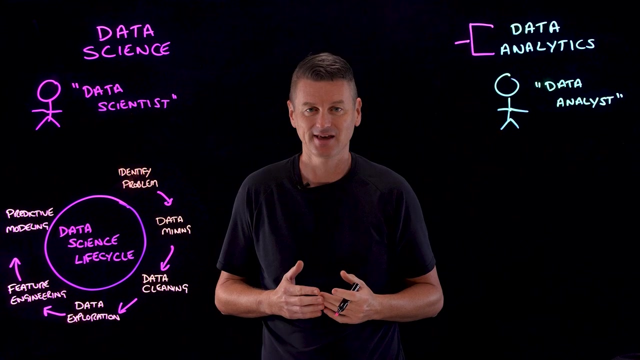 stage, data cleaning, And then at that point we move on to data exploration, analysis to try to make sense of that data. We'll then apply feature engineering, using domain knowledge, to extract details from the data, And predictive modeling comes next, to use the data to predict or forecast future outcomes and behaviors. 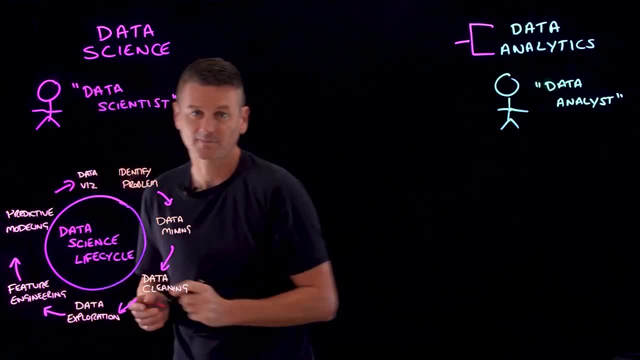 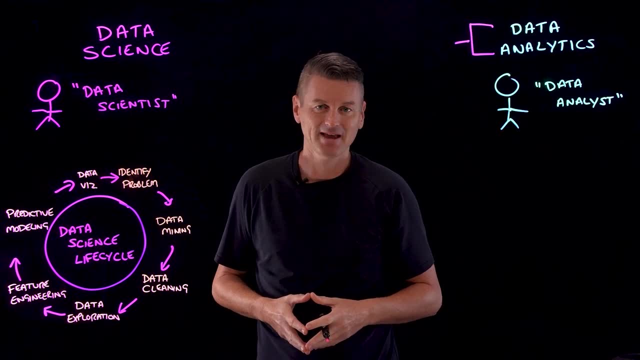 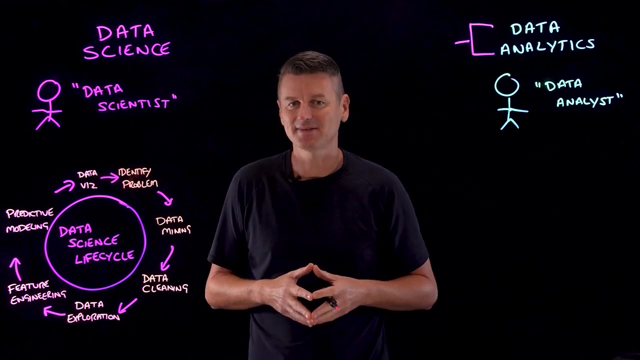 And then, finally, we have data visualization that represents the data points with graphical tools such as charts and animations, and so the life cycle repeats. Now, the role of a data scientist is an in-demand profession right now. If that's something you're interested in, you'll want to develop deep skills in machine learning and AI. 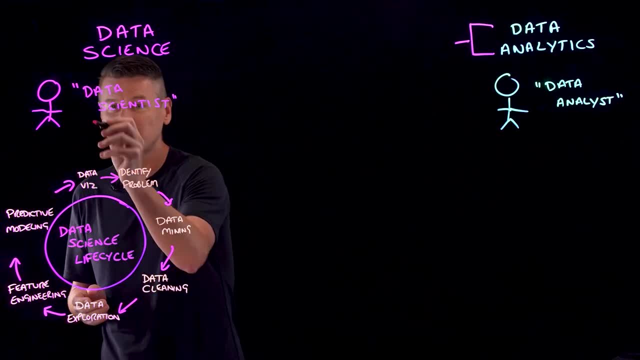 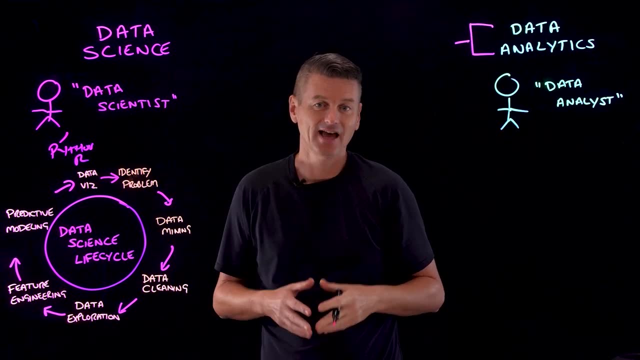 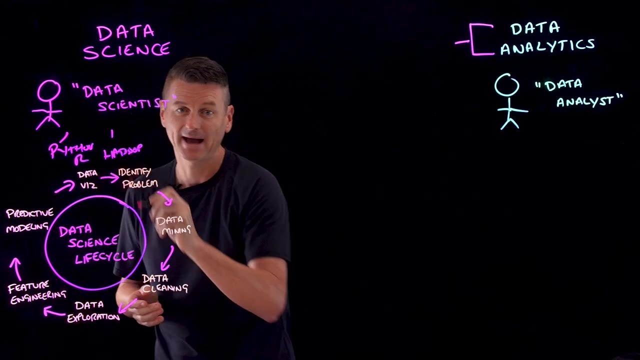 It's helpful to be able to write code in languages such as Python, Also in. R is another popular language for data science, And you should have experience working with big data platforms, so perhaps Hadoop or Apache, Spark, And it's also very helpful to have database knowledge and SQL. 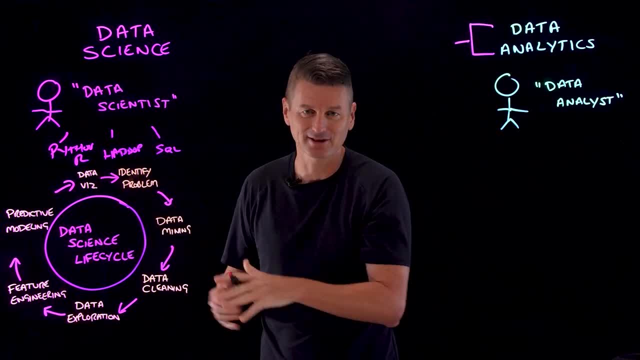 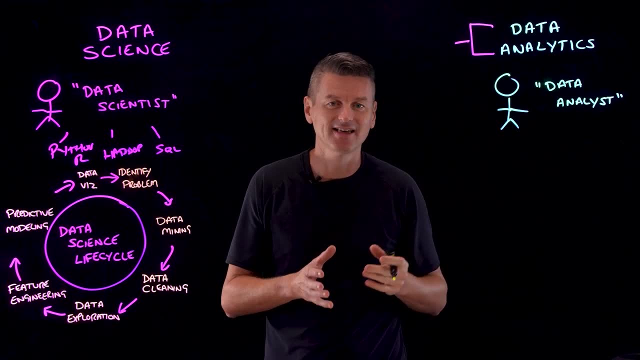 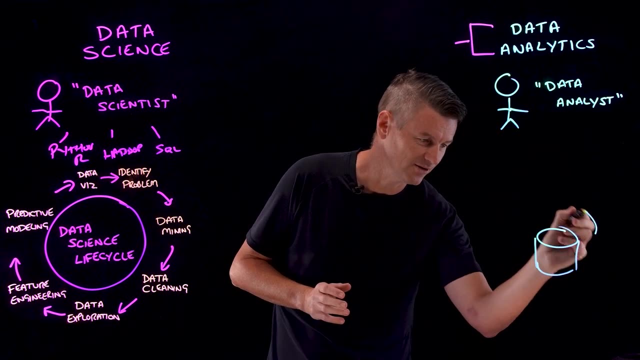 So that's data science, But what about its specialization? data analytics? Well, the job of a data analyst is to conceptualize a data set as it currently exists. So we have some data here and we need to do something with it, And we need to be able to make decisions based on this data. 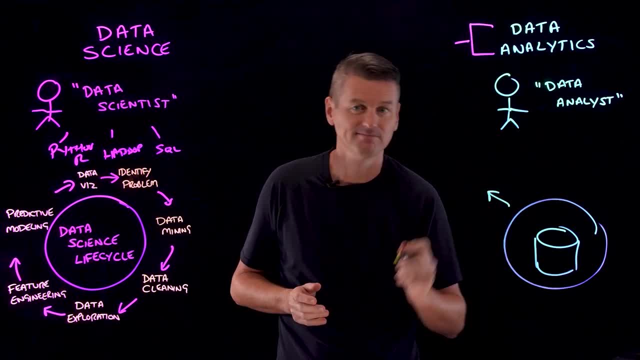 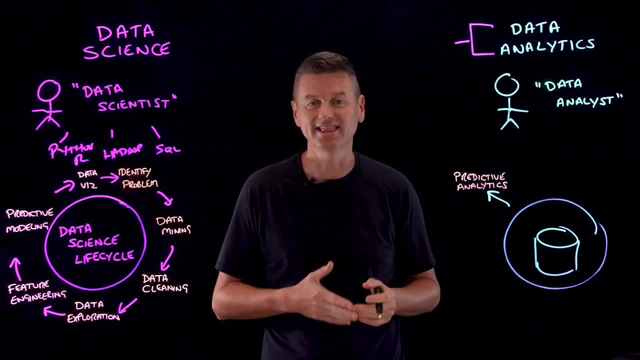 How do we conceptualize it? Well, four ways. One is through predictive analytics. There's predictive analytics, which helps to identify trends, correlations and causation within data sets, like forecasting when those cantaloupes would have all flown off the shelves. 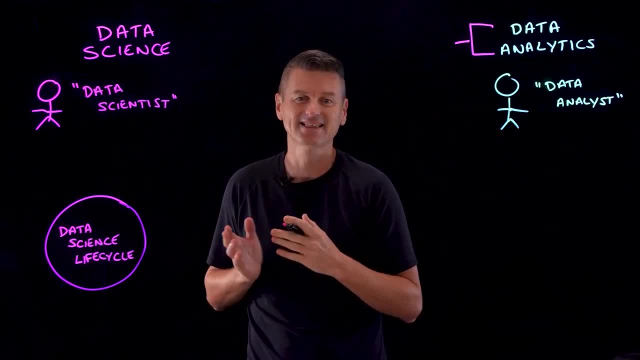 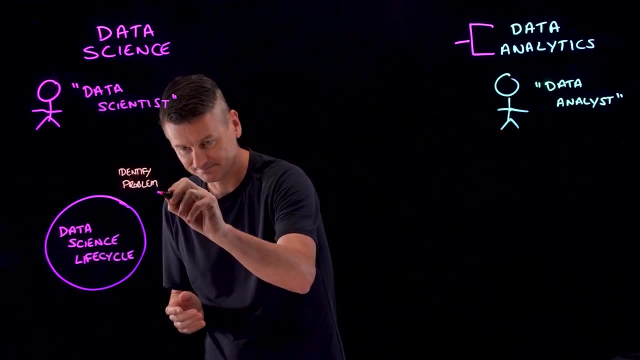 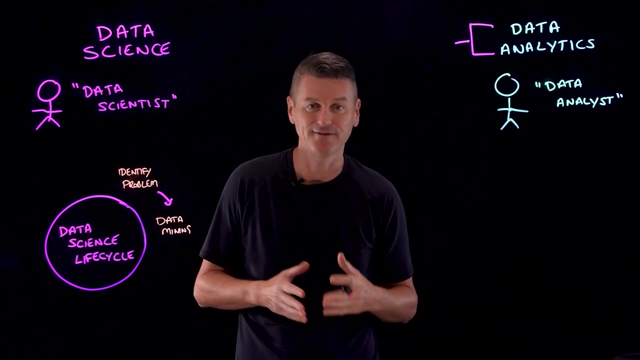 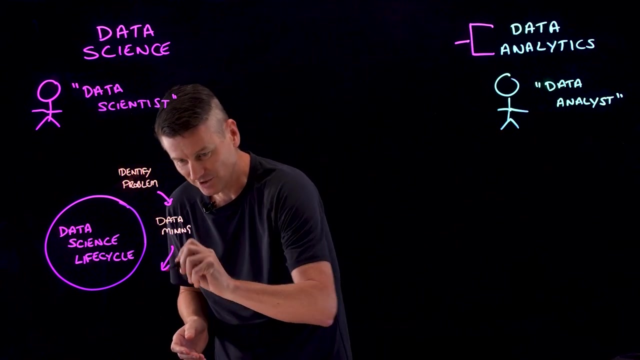 science life cycle, which usually follows seven phases. So first is to identify a problem or an opportunity. Then the next phase is data mining, which is to extract data relevant to that problem or opportunity from large data sets. Now that data will likely consist of a bunch of redundancies and errors, which is fixed in the next. 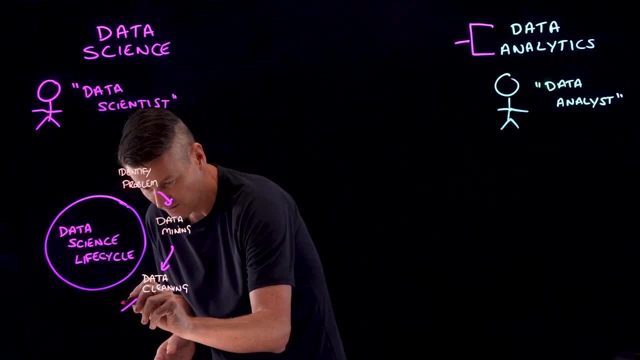 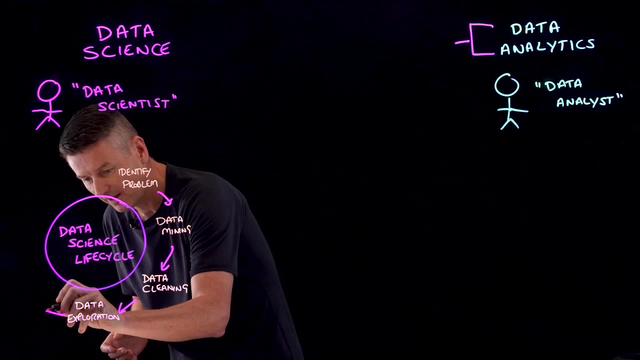 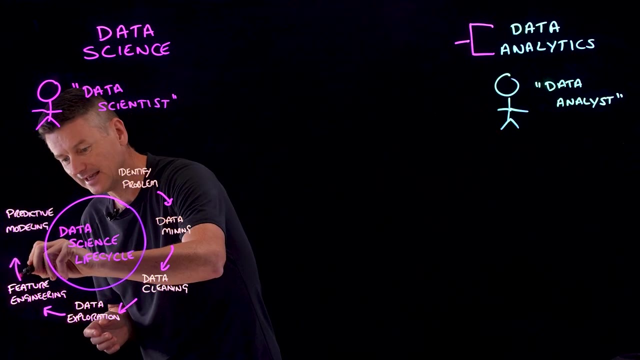 stage, data cleaning, And then at that point we move on to data exploration, analysis to try to make sense of that data. We'll then apply feature engineering, using domain knowledge, to extract details from the data, And predictive modeling comes next, to use the data to predict or forecast future outcomes and behaviors. 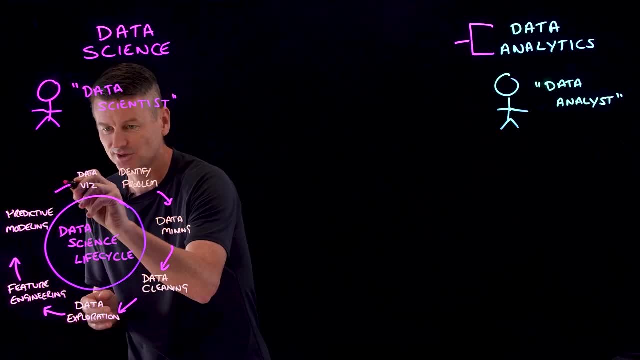 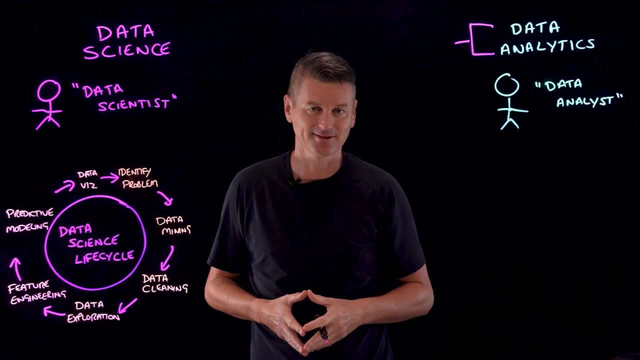 And then, finally, we have data visualization that represents the data points with graphical tools such as charts and animations, and so the life cycle repeats. Now the role of a data scientist is an in-demand profession right now. If that's the case, then it's not a big deal. 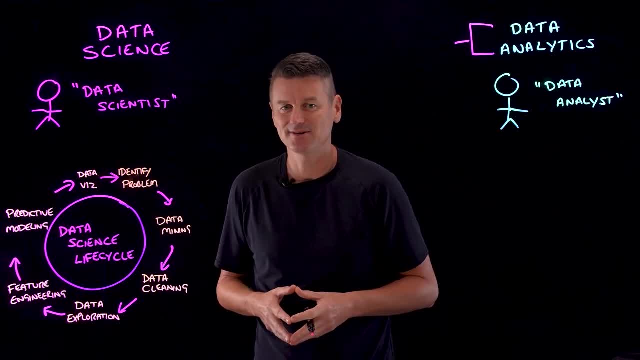 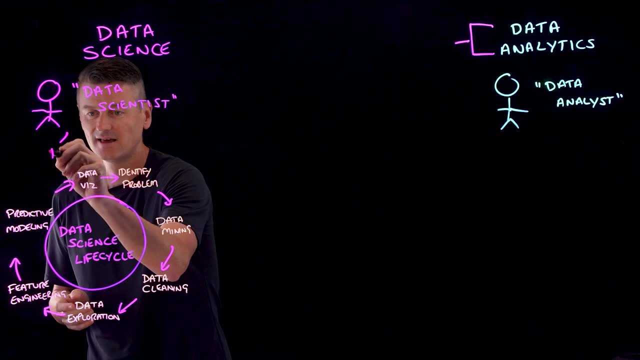 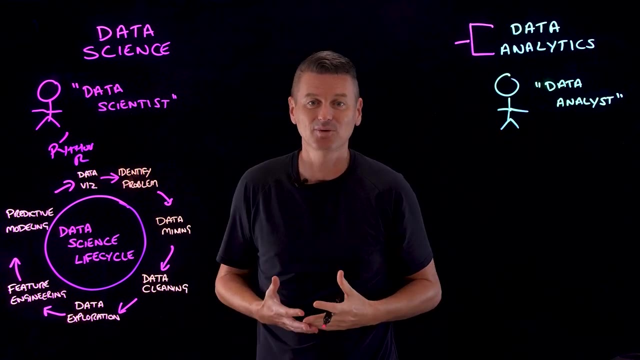 If that's something you're interested in, you'll want to develop deep skills in machine learning and AI. It's helpful to be able to write code in languages such as Python. Also in. R is another popular language for data science, And you should have experience working with big data platforms. 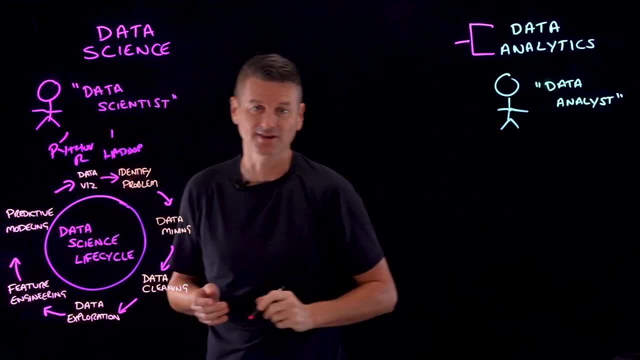 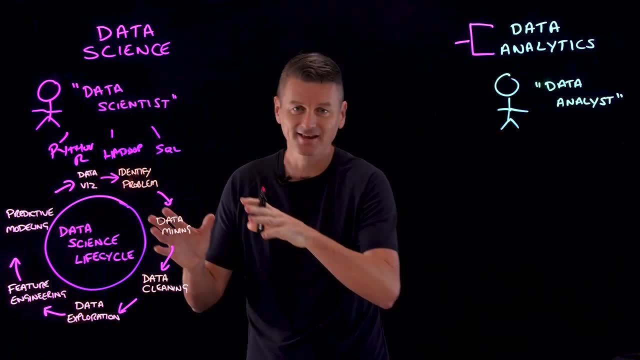 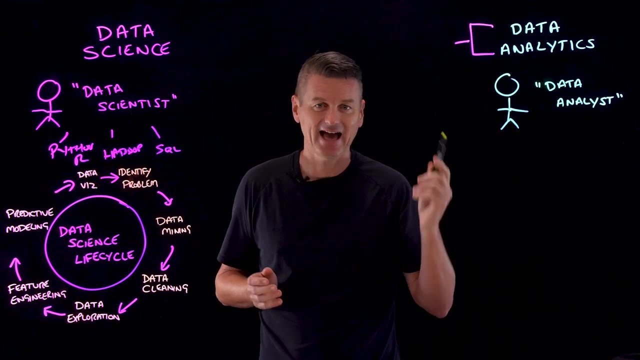 So perhaps Hadoop or Apache Spark, But it's also very helpful to have database knowledge and SQL. So that's data science. But what about its specialization? data analytics? Well, the job of a data analyst is to conceptualize a data set as it currently exists. 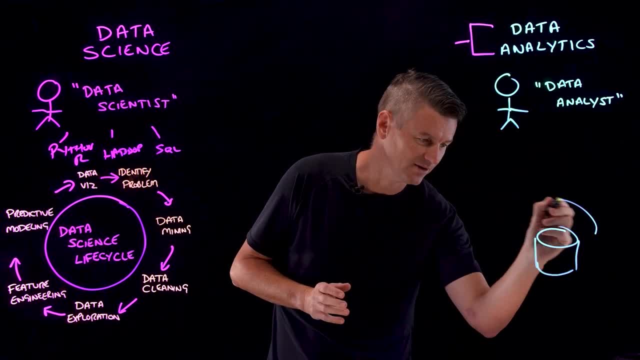 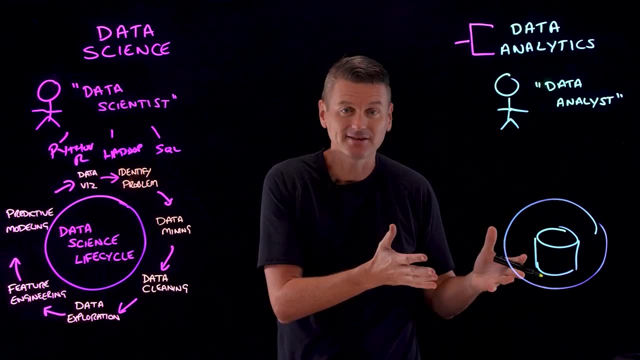 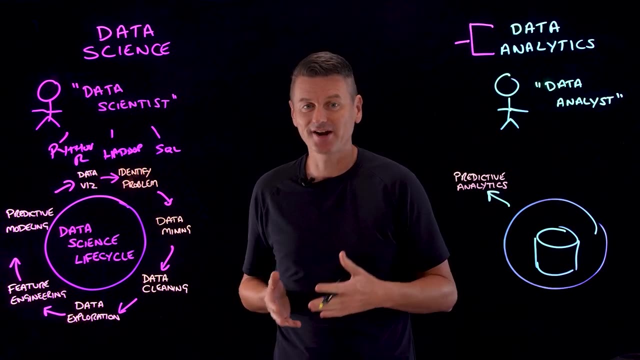 So we have some data here and we need to do something with it And we need to be able to make decisions based on this data. How do we conceptualize it? Well, four ways. One is through predictive analytics, which helps to identify trends, correlations and causation within data sets. 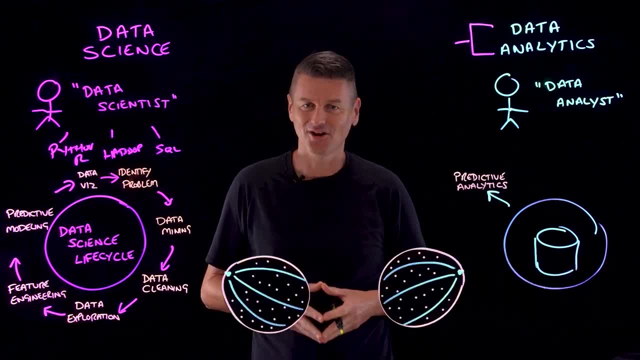 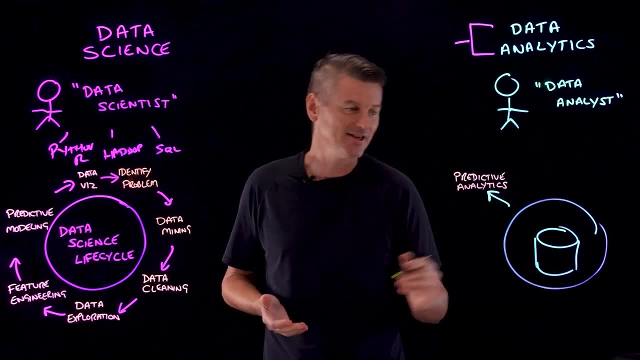 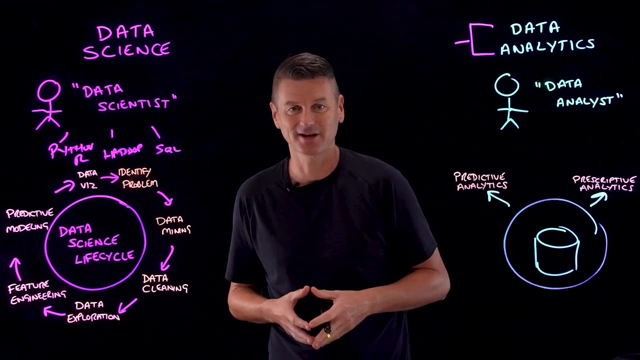 Like forecasting when those cantaloupes would have all flown off the shelves, Or, in healthcare, to forecast regions which will experience a rise in flu cases. There's prescriptive analytics and that predicts likely outcomes and makes decision recommendations, Like predicting when a tire will wear out and need to be replaced. 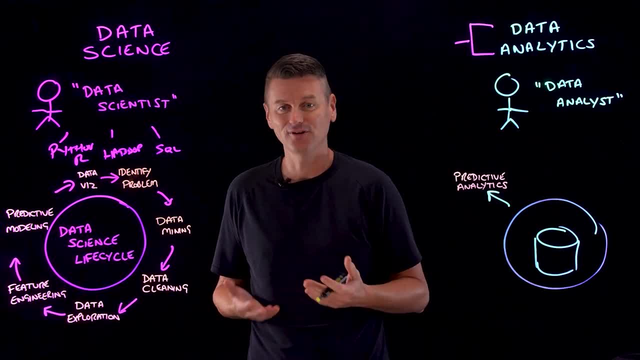 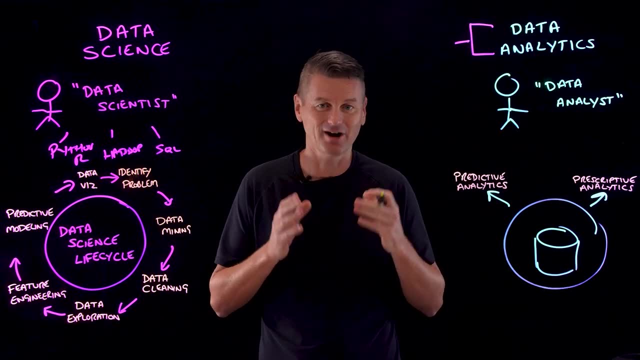 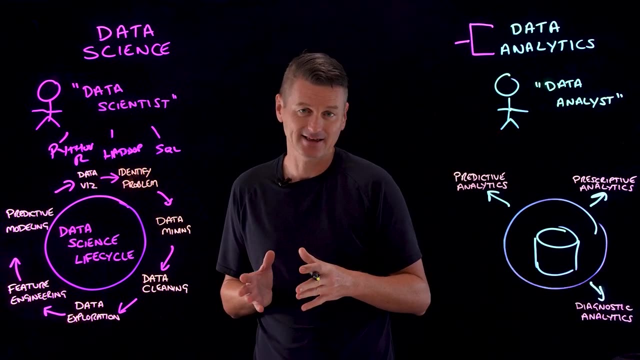 or in healthcare, to forecast regions which will experience a rise in flu cases. There's prescriptive analytics, and that predicts likely outcomes and makes decision recommendations, like predicting when a tire will wear out and need to be replaced. There's diagnostic analytics And that helps pinpoint the reason an event occurred. 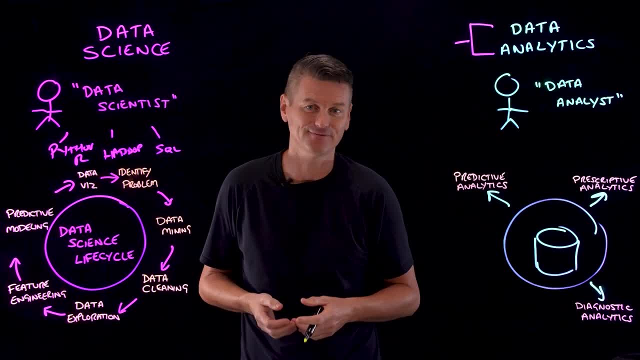 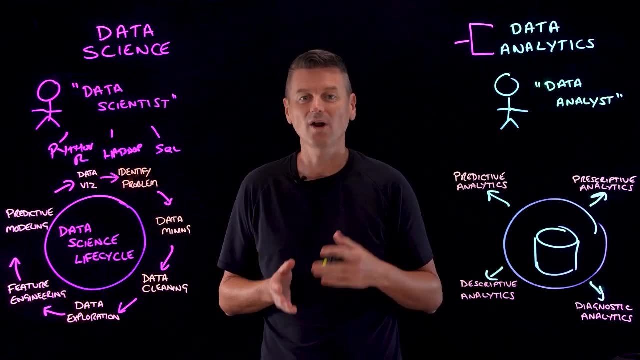 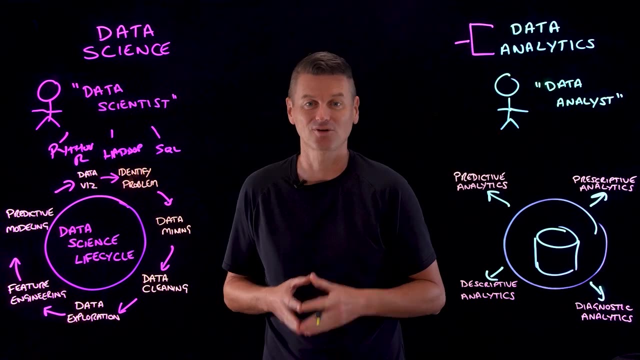 Manufacturers can analyze a failed component on an assembly line and figure out the reason behind its failure. And then there is descriptive analytics, which evaluates the qualities and quantities of a data set. A content streaming provider might use descriptive analytics to understand how many subscribers it's lost. 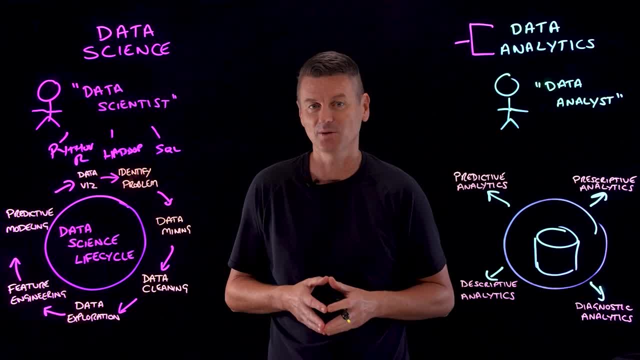 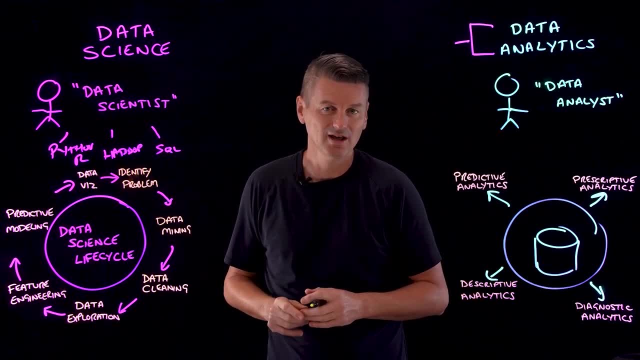 or how many it's gained over a given period of time and what content is being watched. And while a data scientist is a computer scientist, a data analyst is a clearly defined and specialized role. Virtually any stakeholder can be a data analyst. 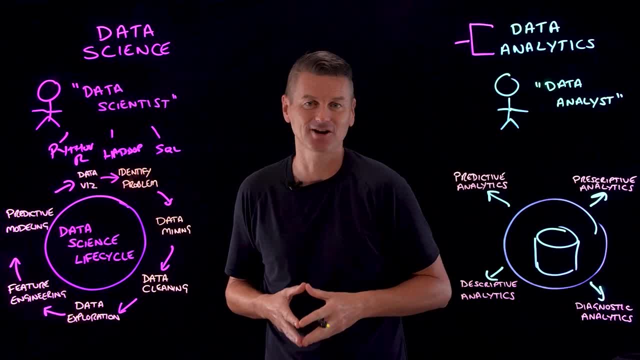 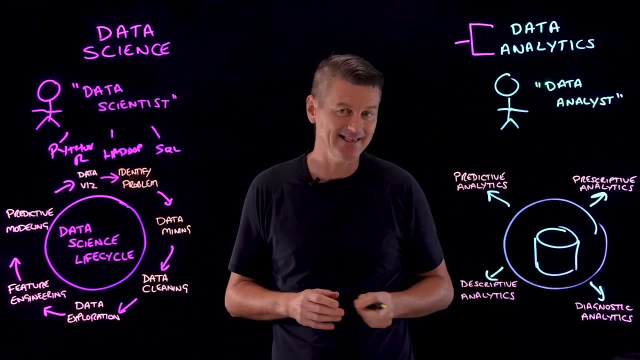 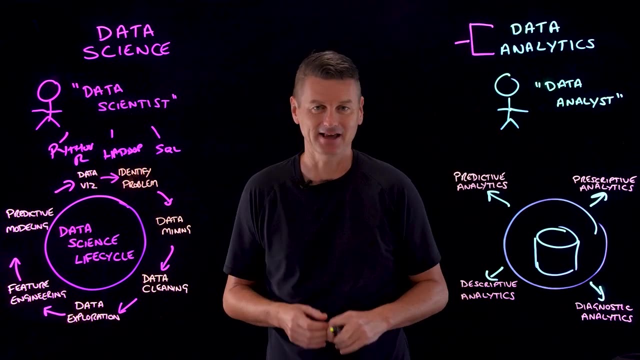 For example, business analysts can use BI dashboards to conduct business analytics and visualize KPIs, But many organizations do employ professional, dedicated data analysts responsible for data wrangling and interpreting findings like why a company's marketing campaign didn't meet expectations. If you want to be a data analyst, 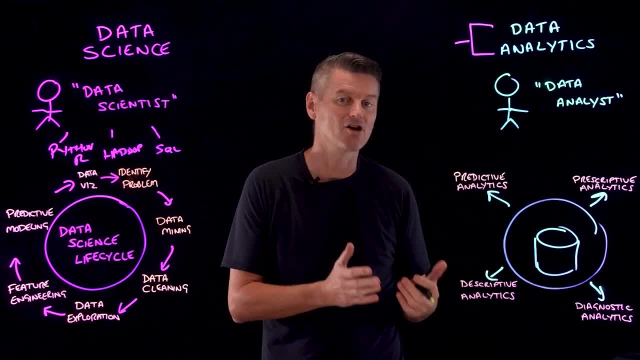 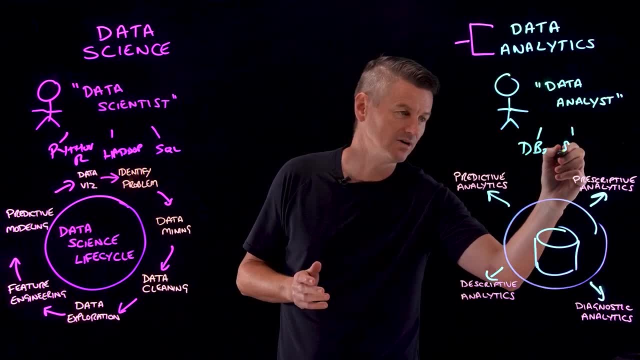 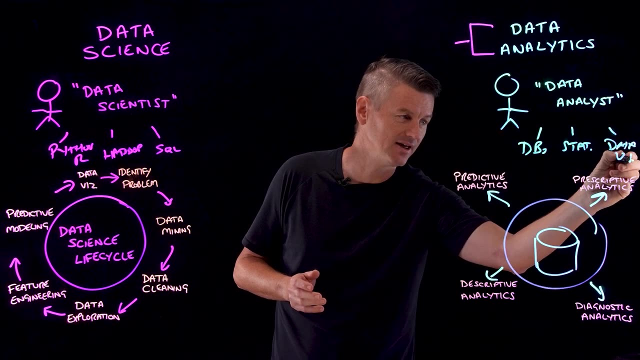 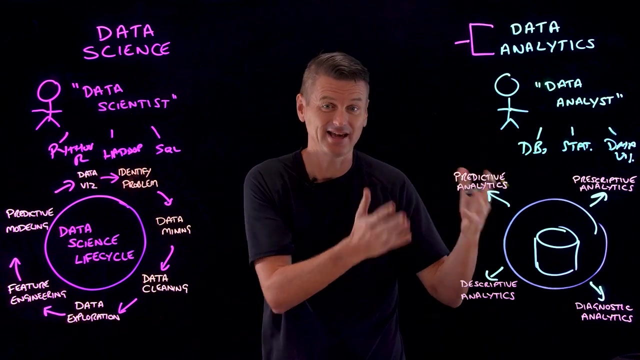 it helps to have both analytical and programming skills, So this includes familiarity with databases. Also, you'll need to know about statistical analysis, and also data visualization is another important skill. So data analytics is often more focused on using statistical tools and techniques to interpret existing data and offer actionable insights. 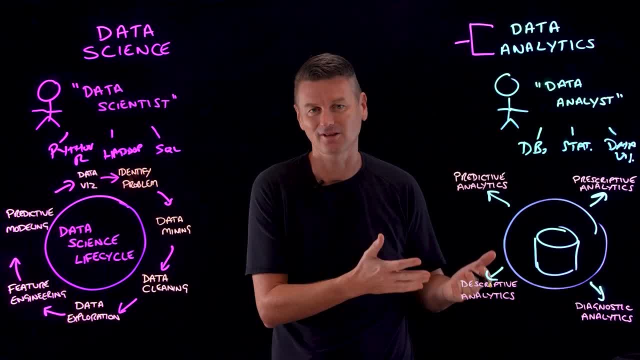 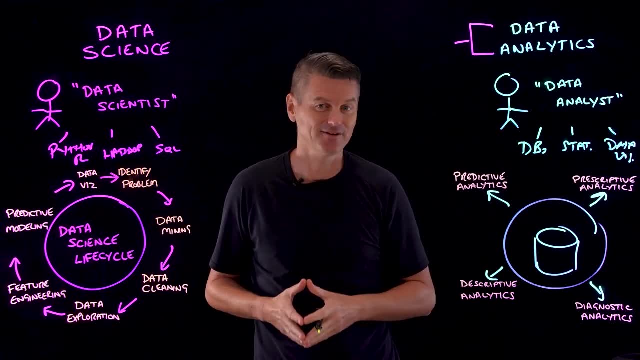 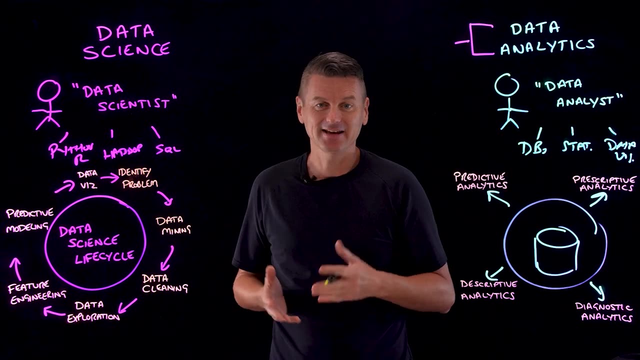 It's usually less concerned with creating new algorithms or models. Data science, on the other hand, has a broader scope that can involve complex machine learning algorithms often created from scratch. Data science focuses on phases from data collection to predictive modeling. Data analysis, on the other hand, is more about answering specific questions with that data. 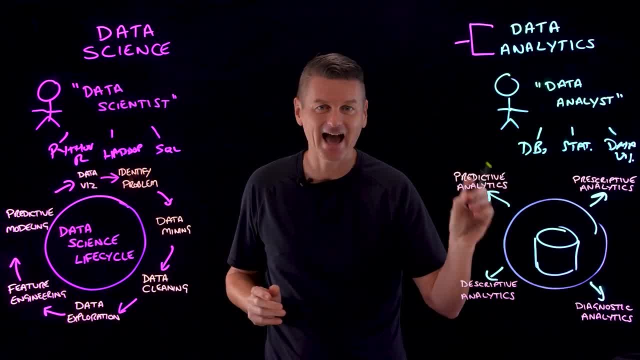 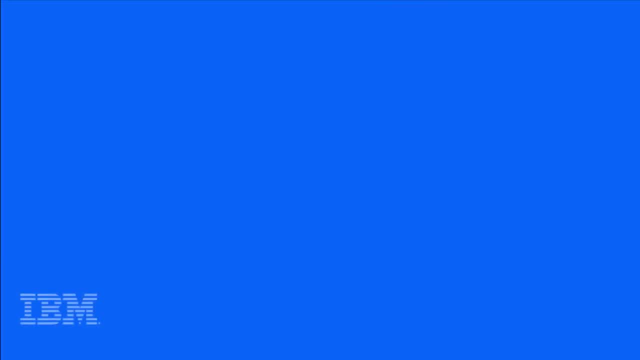 And if you've done both your data science and data analytics right, you'll always be able to keep cantaloupes and just about everything else in stock. 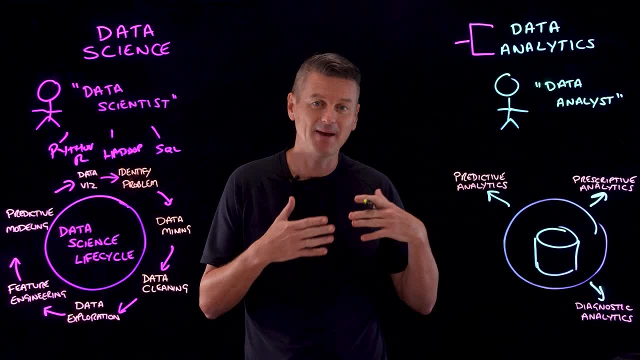 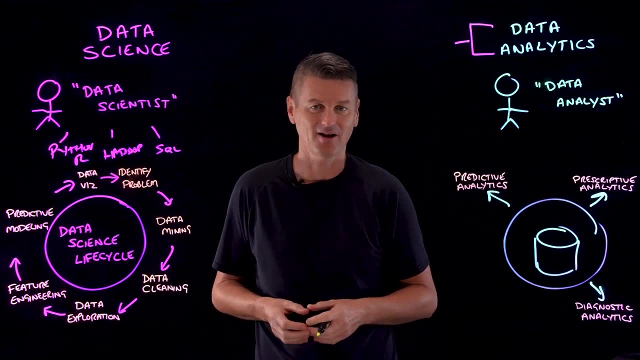 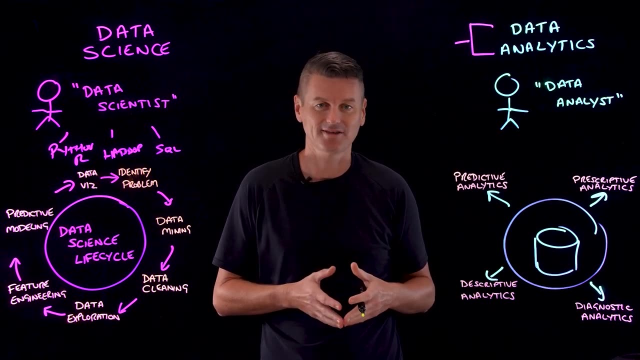 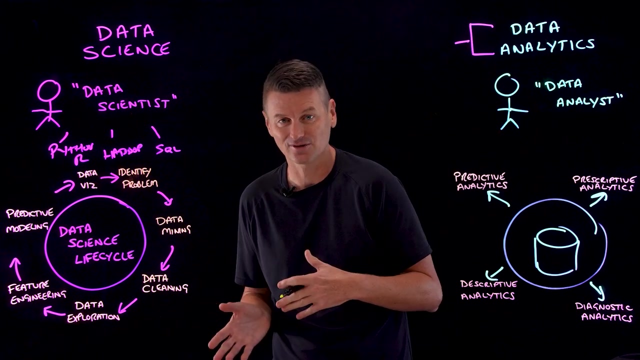 There's diagnostic analytics that helps pinpoint the reason an event occurred. Manufacturers can analyze a failed component on an assembly line and figure out the reason behind its failure. And then there is descriptive analytics, which evaluates the qualities and quantities of a data set. A content streaming provider might use descriptive analytics to understand how many subscribers it's lost. 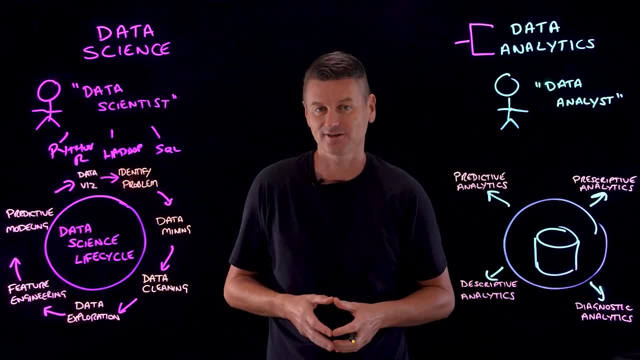 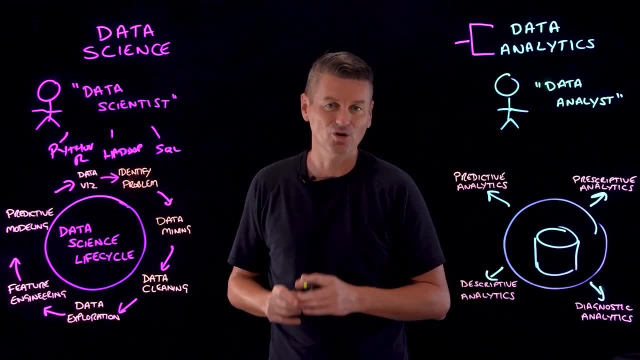 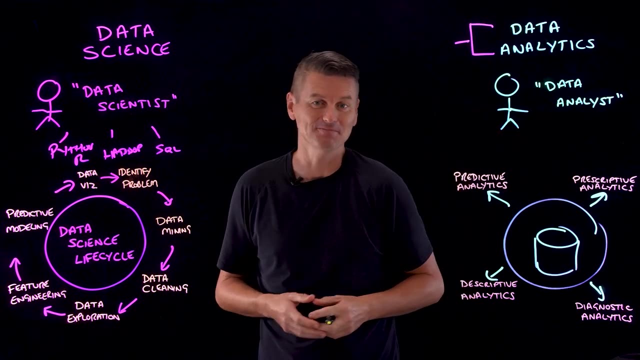 or how many it's gained over a given period of time and what content is being watched. And while a data scientist is a clearly defined and specialized role, virtually any stakeholder can be a data analyst. For example, business analysts can use BI dashboards to conduct business analytics and visualize KPIs. 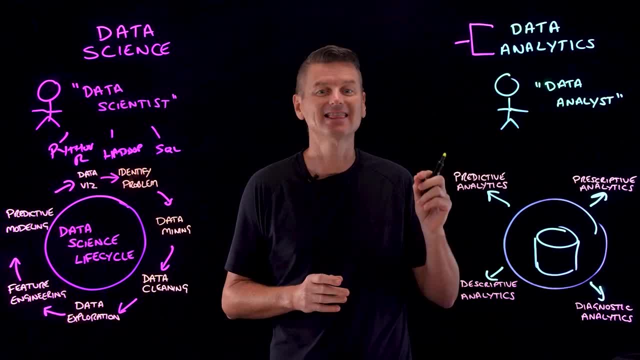 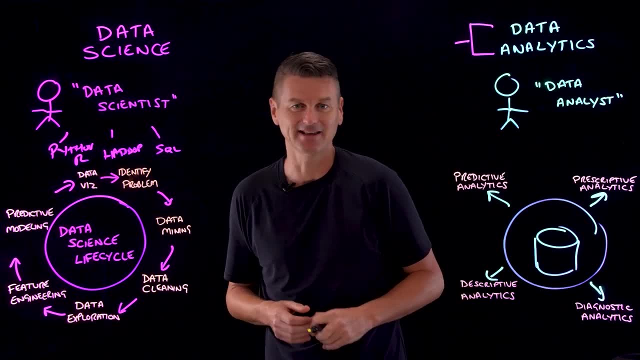 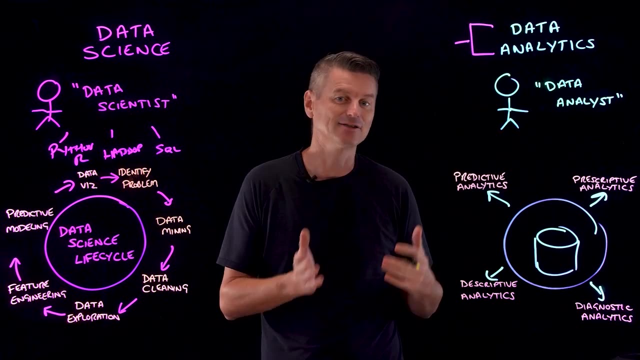 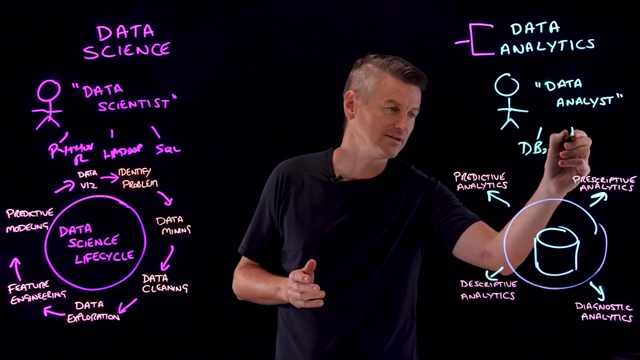 But many organizations do employ professional, dedicated data analysts responsible for data wrangling and interpreting findings, like why a company's marketing campaign didn't meet expectations. If you want to be a data analyst, it helps to have both analytical and programming skills, So this includes familiarity with databases. also, you'll need to know about statistical analysis. 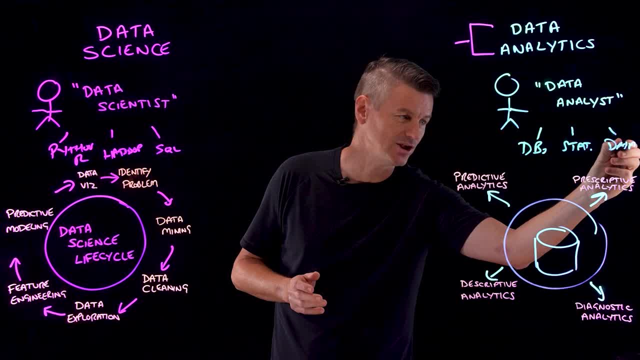 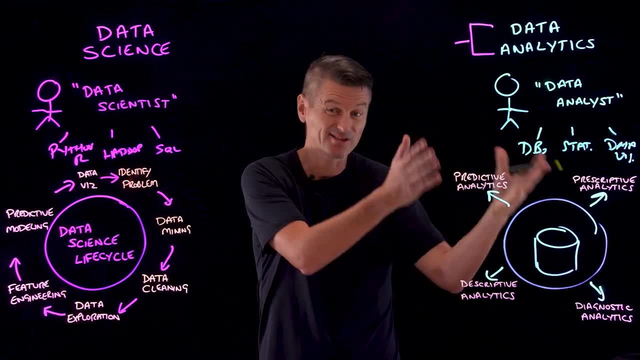 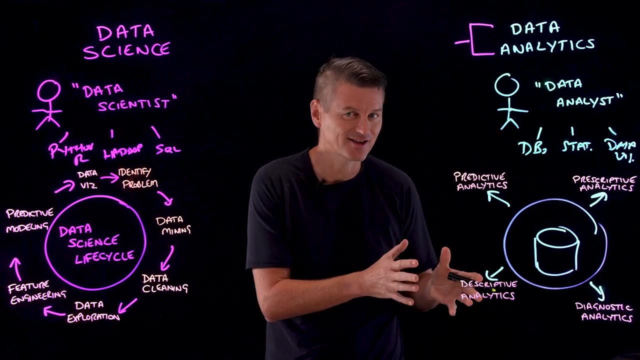 and also data visualization is another important skill. So data analytics is often more focused on using statistical tools and techniques to interpret existing data and offer action, actionable insights. It's usually less concerned with creating new algorithms or models. Data science, on the other hand, has a broader scope that can involve complex 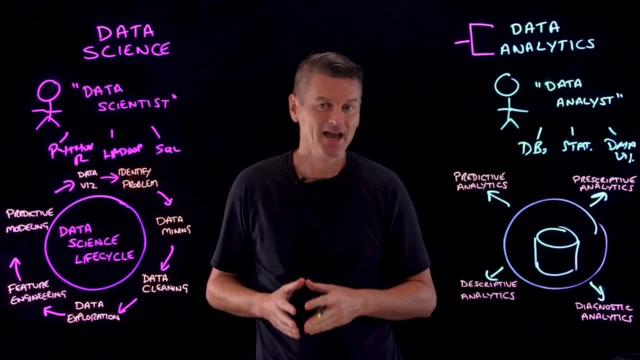 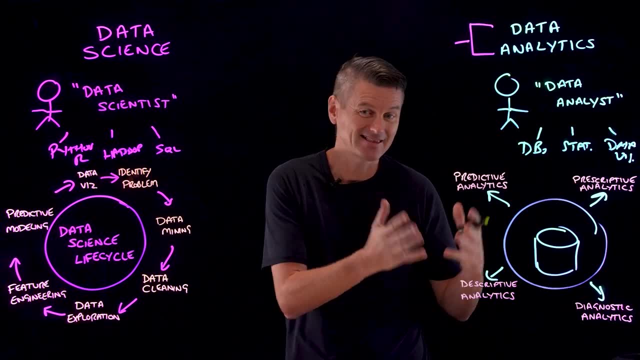 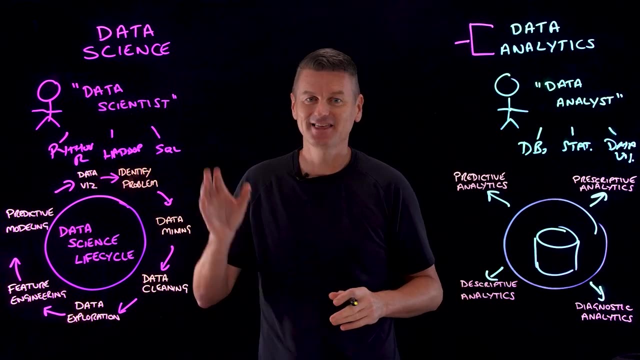 machine learning algorithms, often created from scratch. Data science focuses on phases from data collection to predictive modeling. Data analysis, on the other hand, is more about answering specific questions with that data, And if you've done both your data science and data analytics right, you'll always 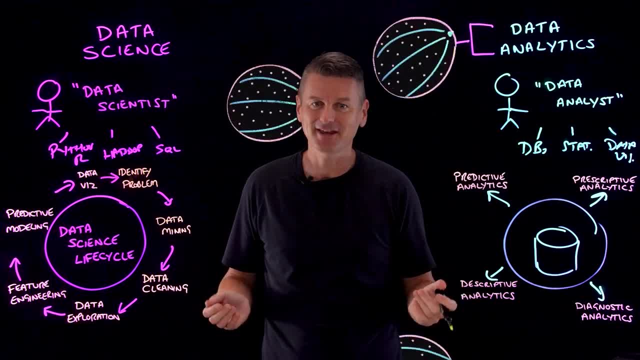 be able to keep cantaloupes and just about everything else in stock. 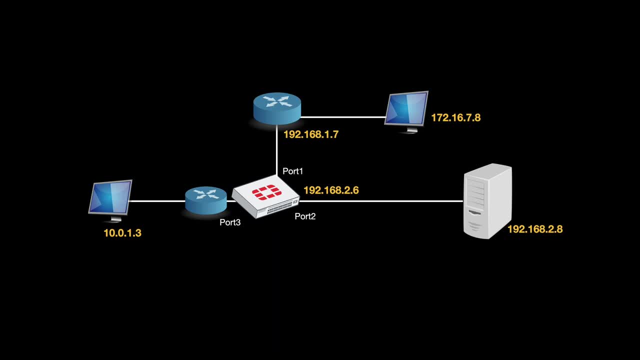 A key routing concept on your FortiGate is RPF- reverse path forwarding. It is a mechanism that protects you from IP spoofing, and it works like that. Any packet that is sent towards your network is checked. If there's a route towards the source IP, the packet will continue to its destination.